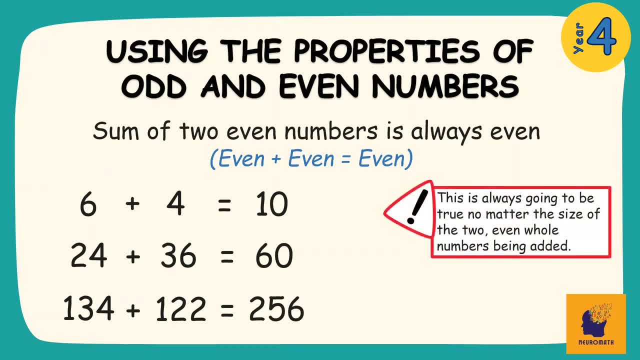 What's also important to remember is that this condition is always going to be true, no matter if I have two even numbers added. So even if I have something like a 6-digit even number being added with a 3-digit even number, my answer will still be an even number. 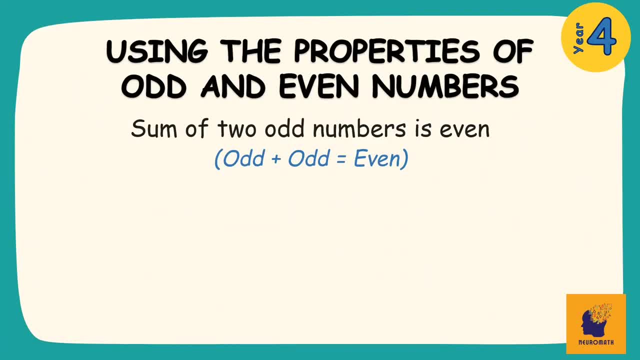 The next thing we need to understand is that the sum of two odd numbers is always going to be even. What this means is that when I add two odd numbers together, I will get an even number as a result. So if I have something like this, I will get an even number as a result. So if I have something 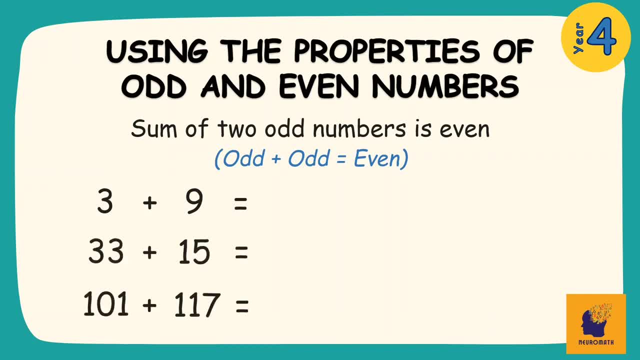 like 3 plus 9, or 33 plus 15, or 101 plus 117,, because they're two odd numbers being added together. I will get an even number as an answer And again we can check that this condition is. 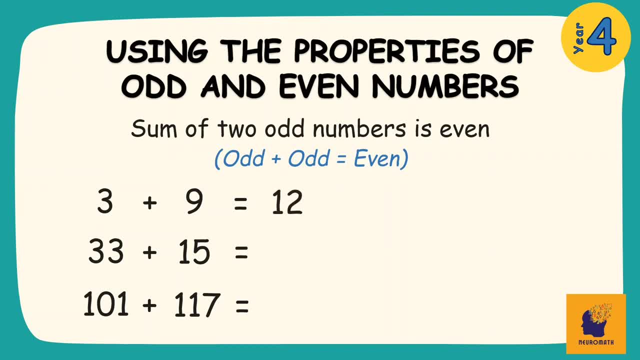 true, 3 plus 9 being 12,, which is an even number, 33 plus 15 being 48,, which is an even number, and 101 plus 117 being 218,, which is an even number. Like the previous condition, this is always going to be true, no matter the size of the two. 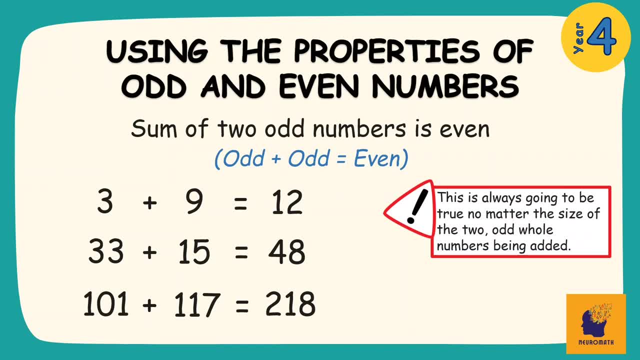 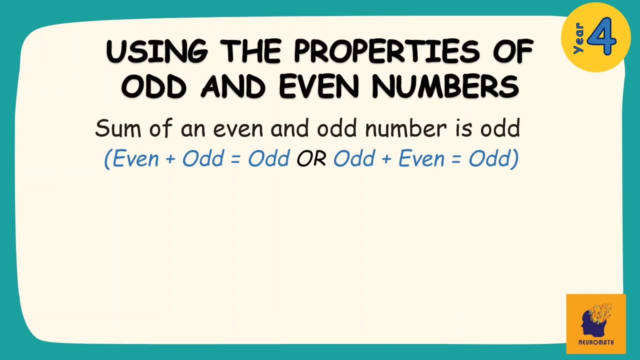 odd whole numbers being added, So I could have an odd number that is three digits long being added to an odd number that is five digits long. My answer will still be an even number. The last thing we need to understand is that the sum of an even and an odd number 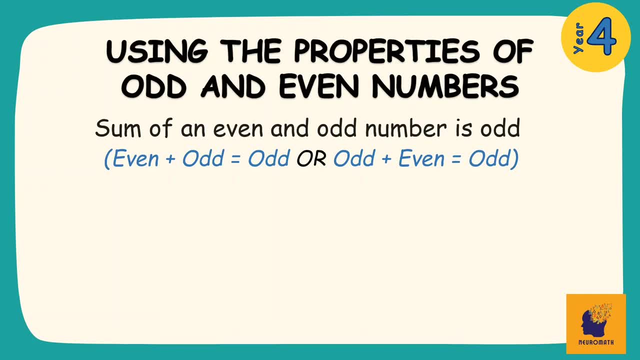 is always going to be odd. What this means is that when I add two odd numbers together and add an even and an odd, or an odd and an even, I will get an odd number as my answer. So I could have problems like 8 plus 5,, 17 plus 24, or 156 plus 115.. Because an odd number 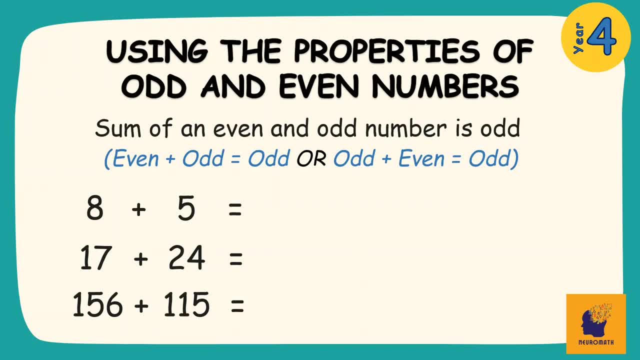 is being added with an even number. I will get an odd number as my answer And, like with the previous conditions, we can check that this is true by solving our problems: 8 plus 5 being 13,- an odd number, 17 plus 24 being 41, an odd number And 156 plus 115.